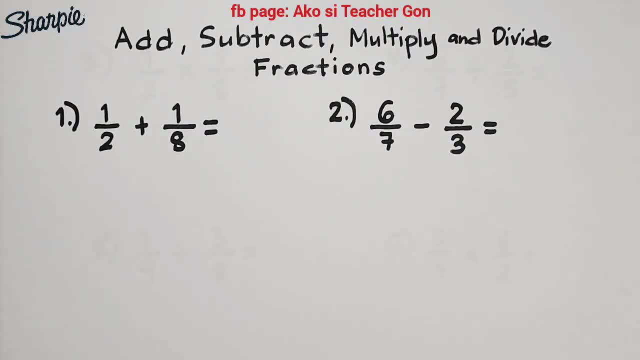 Hi guys, it's me, Teacher Gon. In today's video, we will talk about how to add, subtract, multiply and divide fractions. So, without further ado, let's do this topic. So I have prepared six different examples for this video, and let's try number one. 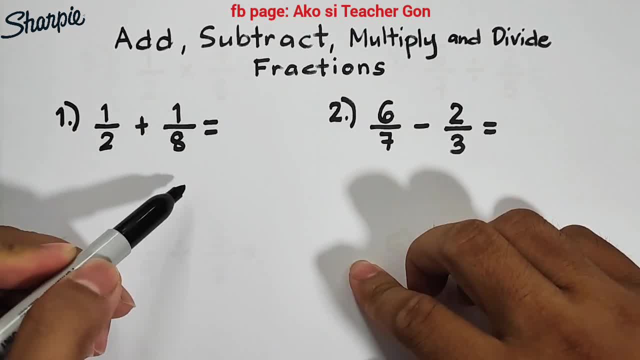 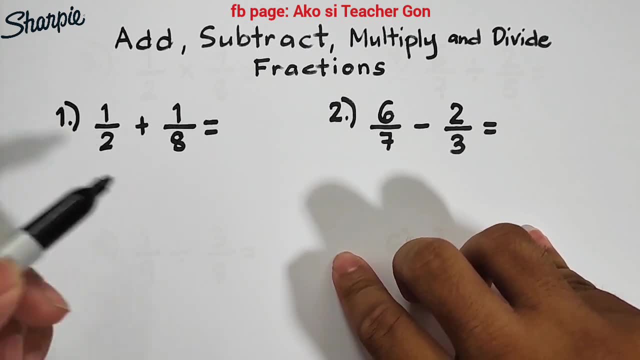 In number one we have 1 half plus 1 over 8. So to add these two fractions, first we need to find the LCD. The denominators are 2 and 8. So the target we have here is to find the LCD. 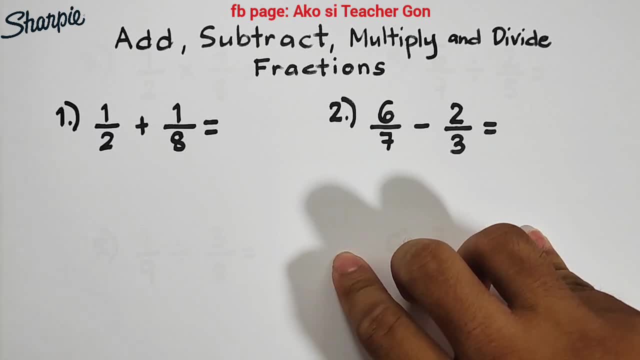 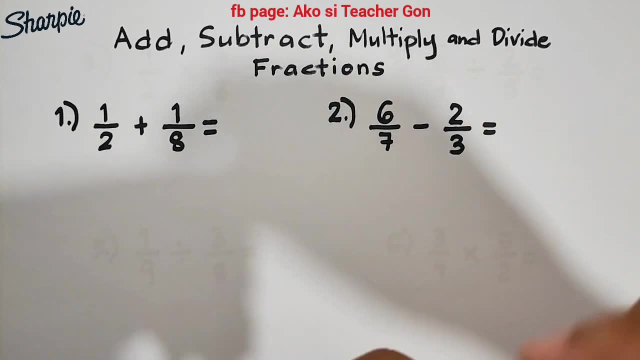 So there are different ways on how to find the LCD. Some of them are using listing method. Again, one more time, Take two. Hi guys, it's me Teacher Gon. In today's video, we will talk about how to add, subtract, multiply and divide fractions. 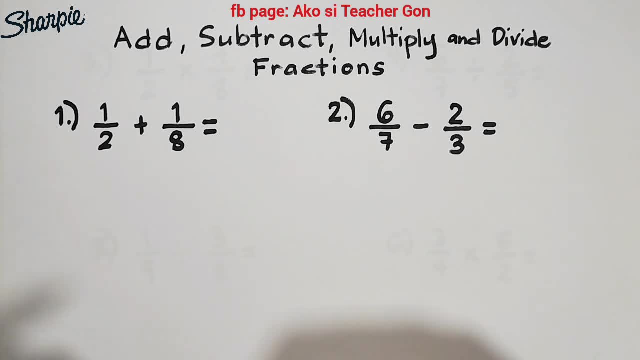 So from the previous comments that I have read from our different videos, they are asking if we could create a video wherein the addition, subtraction, multiplying and dividing fractions are combined. So I have six different examples here And we will try to find the LCD. 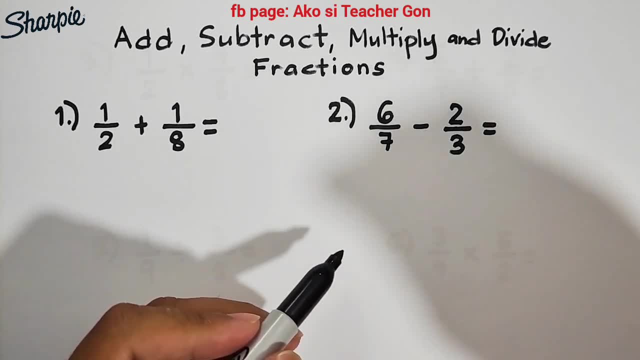 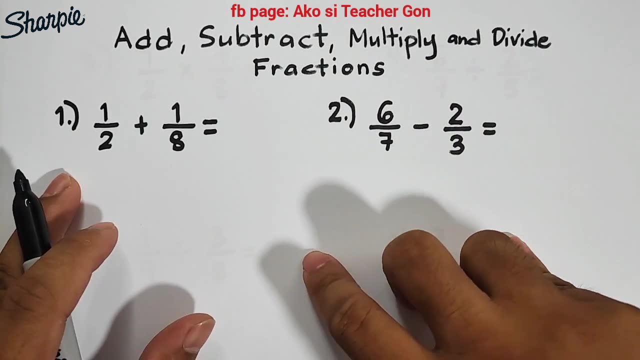 So we will try to answer the four different examples, and the last two will be your task in solving or after this video. So let's start with number one. In number one, we are asked: what is 1 half plus 1 over 8?? 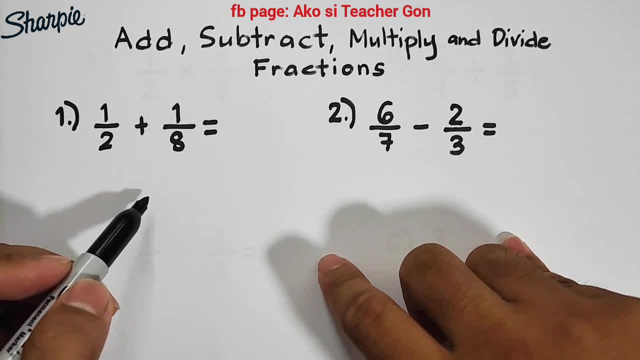 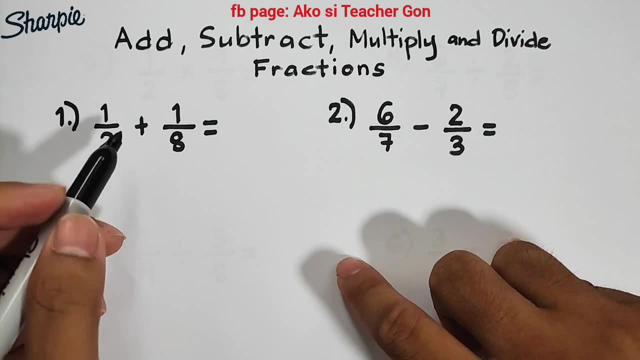 So this one is addition. So what we need to do here first is to find the least common denominator. We have denominators which is 2 and 8, which is different, So what we need to do here is to find the least common denominator. 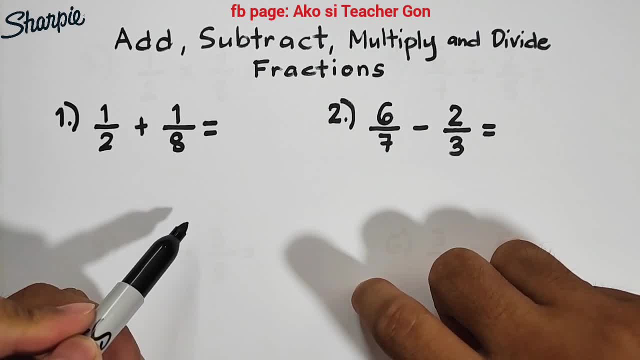 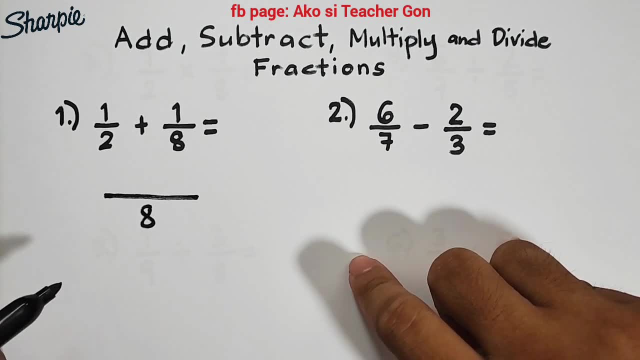 So, given this 2 and 8,, the least common denominator is 8.. So we can put here all over 8.. Now, sir, how do we get the least common denominator? You can use the listing method to get the LCM of 2 and 8.. 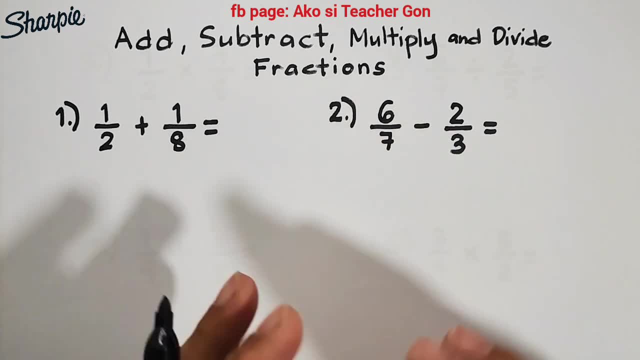 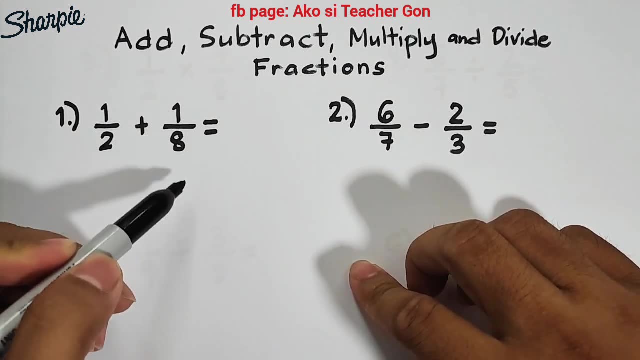 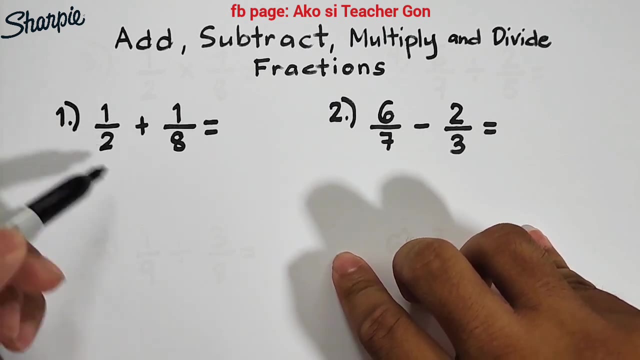 So, I have prepared six different examples for this video, and let's try number one. In number one, we have 1 half plus 1 over 8. So, to add these two fractions, first, we need to find the LCD. The denominators are 2 and 8. So, the target we have here is to find the LCD. So, there are different ways on how to find the LCD. Some of them are using listing method. Again, one more time. Take two. 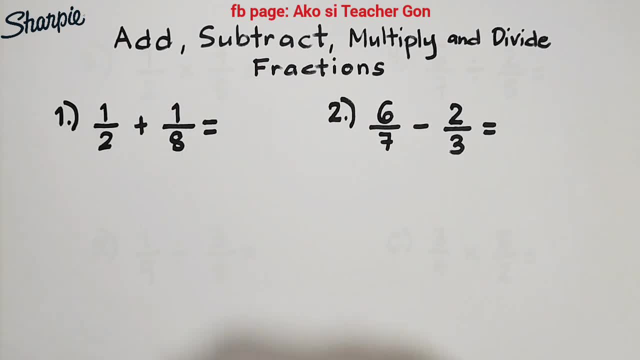 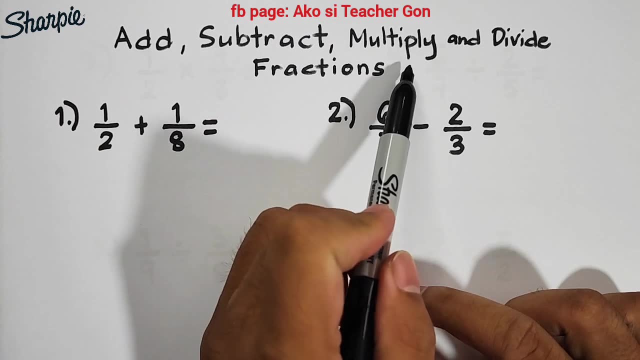 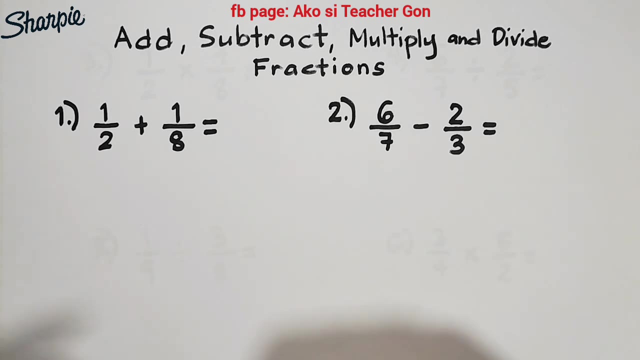 Hi guys, it's me, Teacher Gon. In today's video, we will talk about how to add, subtract, multiply, and divide fractions. So, from the previous comments that I have read from our different videos, they are asking if we could create a video wherein the addition, subtraction, multiplying, and dividing fractions are combined. So, I have six different examples here. And we will try to find the LCD. So, I will try to answer the four different examples, and the last two will be your task in solving or after this video. 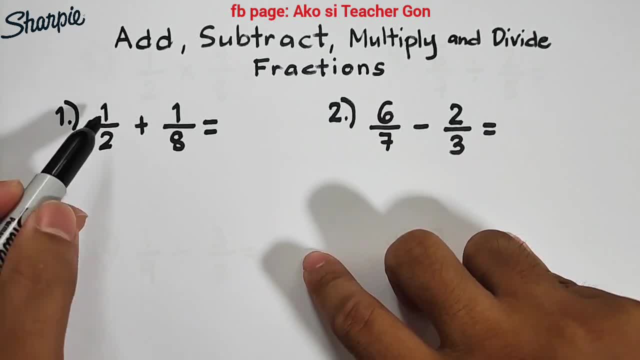 So, let's start with number one. In number one, we are asked, what is 1 half plus 1 over 8? So, this one is addition. 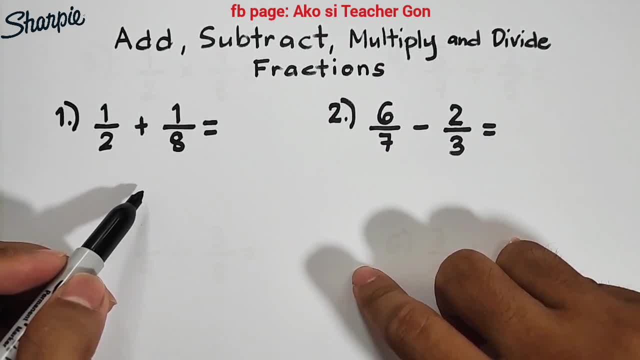 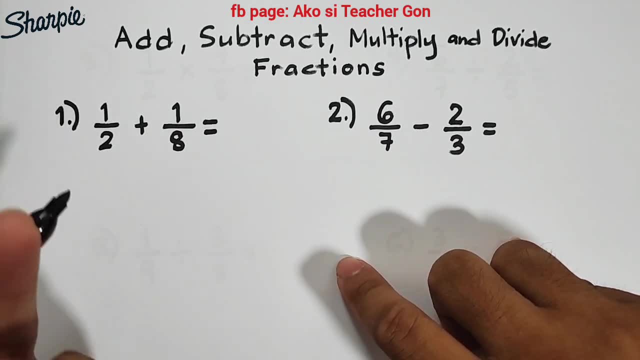 So, what we need to do here, first, is to find the least common denominator. We have denominators, which is 2 and 8, which is different. So, what we need here is to find the least common denominator. So, given this 2 and 8, the least common denominator is 8. So, we can put here, all over 8. Now, sir, how do we get the least common denominator? You can use a listing method to get the LCM of 2 and 8. 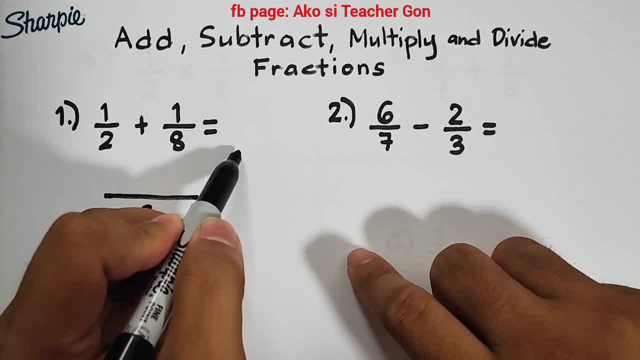 So, when you list it, it will become like this. I will show it to you. 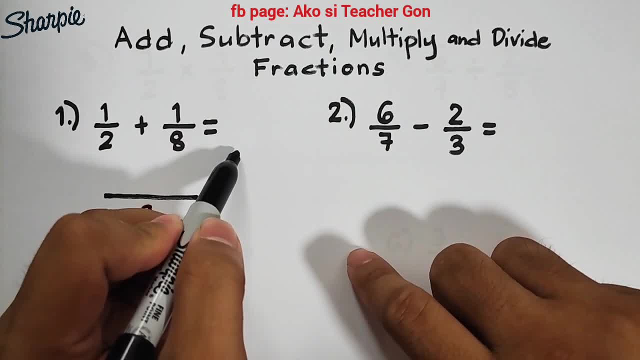 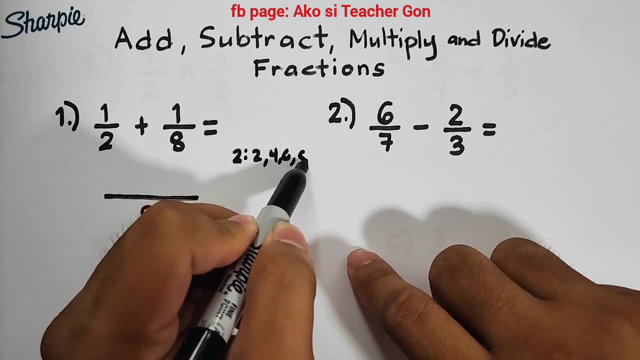 So when you list it, it will become like this. I will show it to you: 2, 4,, 5,, 6,, 7, 8.. 2, 4, 6,, 8,, 16, and so on. 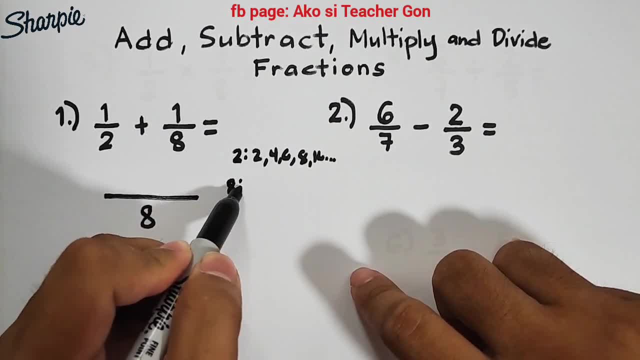 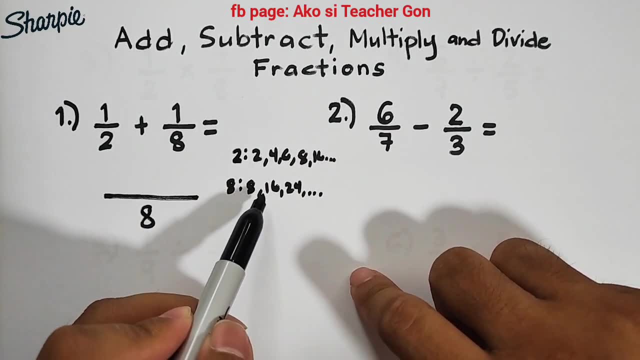 We are just listing the multiples of 2. And for 8,, so we have 8,, 16,, 24, and so on. As you can see, we have common multiples here, which is 8.. Yes, sir, we also have 16.. 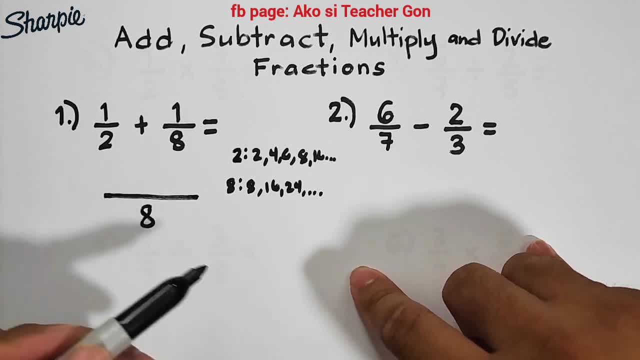 Ah, that's not it, Because our target here is to get the least common multiple, which is equal to 8.. And then this least common multiple is 8.. So 8 will serve as your LCD, or your least common denominator. 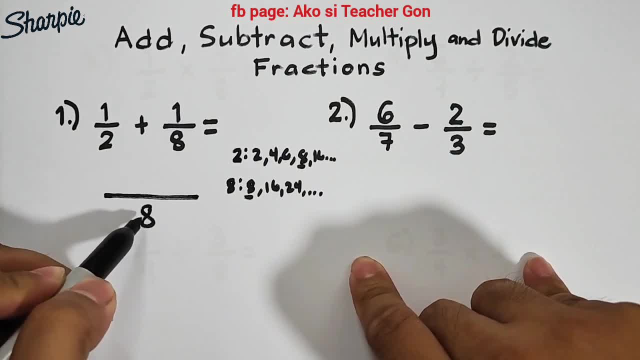 So what's next Is this least common denominator. we need to divide it here in the original denominator, which is 8 divided by 2, that is equal to 4.. And then multiply: 8 divided by 2 is 4.. 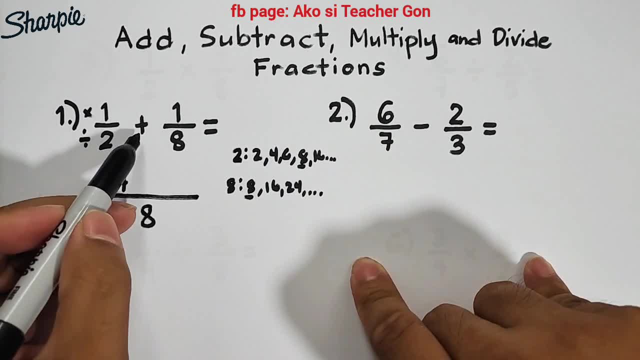 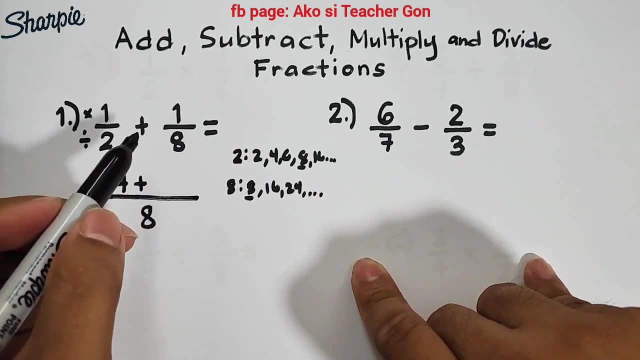 Times 1,, we have now 4. Plus 8 divided by 8, which is equal to 1.. And then multiply 8 divided by 2 is 4. Times 1,, that is equal to 1.. 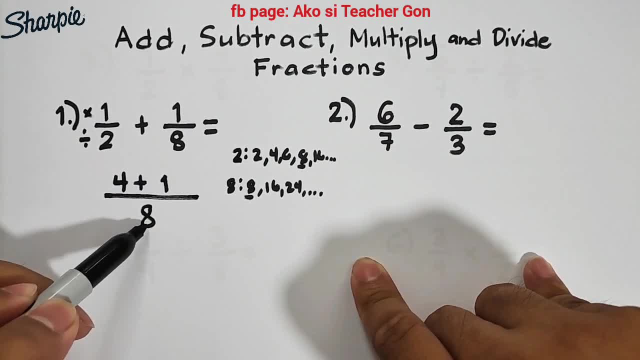 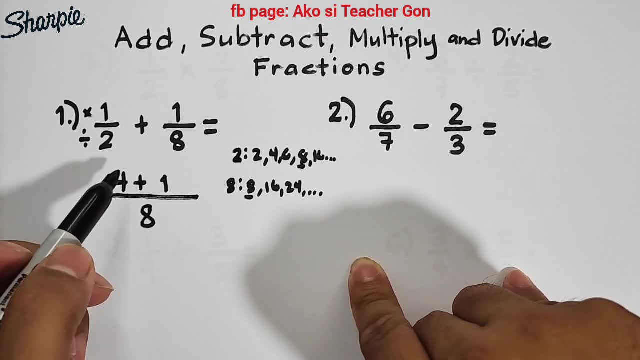 Again. let me repeat the process. First, you will divide this LCD to your original denominators and then multiply it to the numerator. So what we have now is 4 plus 1 over 8, and we need to simplify this. 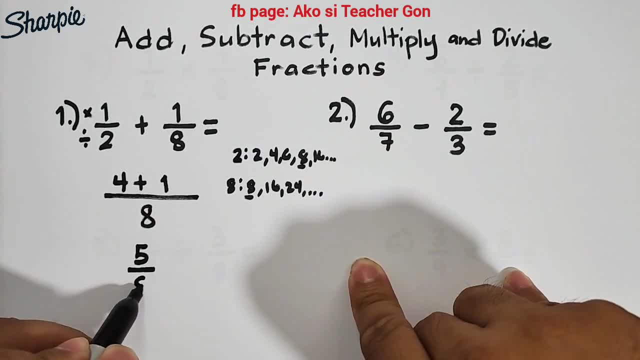 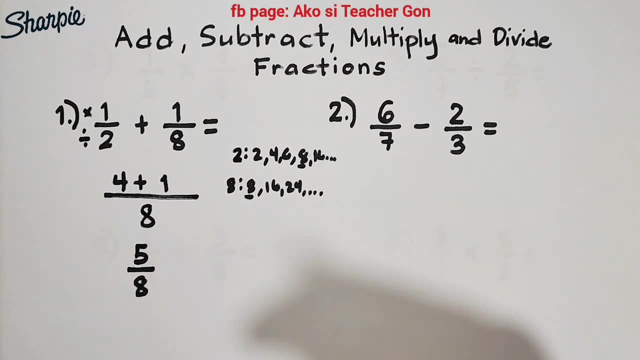 And the answer here is 5 over 8.. By the way, guys, before declaring that your answer is the final answer, you need to check if the given fraction is already in simplified form. So how will we know if it's already simplified, if it doesn't have a common factor? 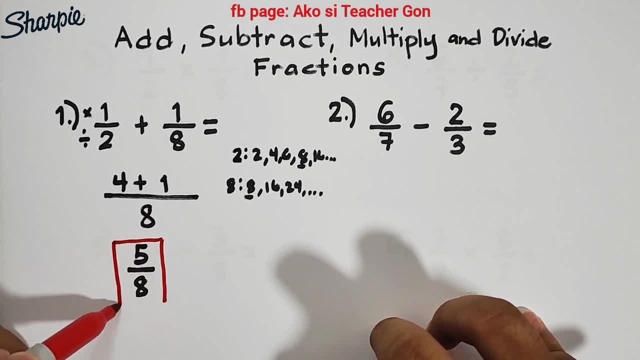 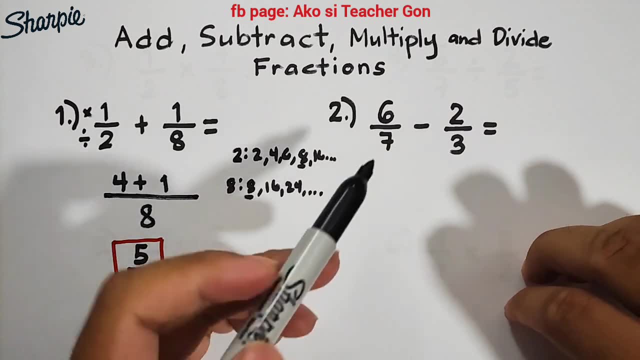 Okay, So therefore this is the final answer: We have 5 over 8.. Now let's move on with item number 2.. For number 2, we have 6 over 7 minus 2 over 3.. 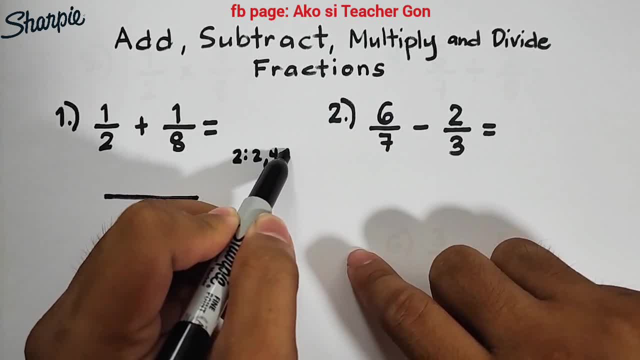 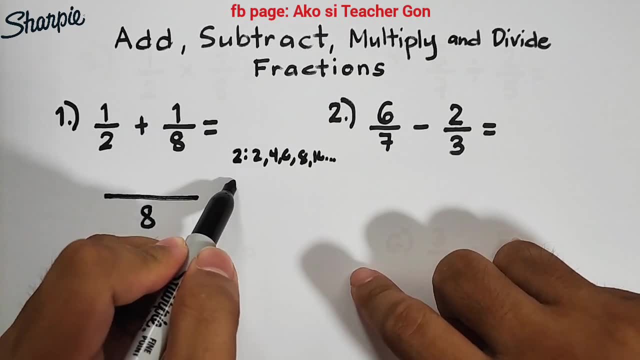 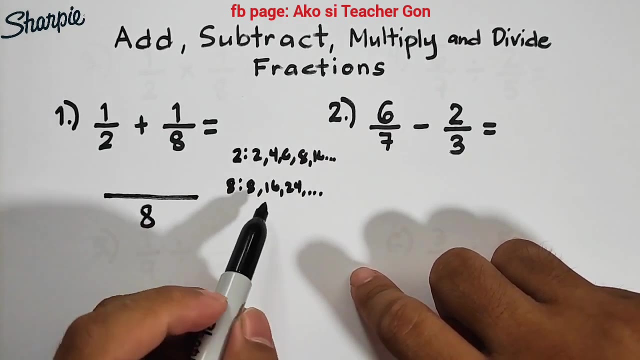 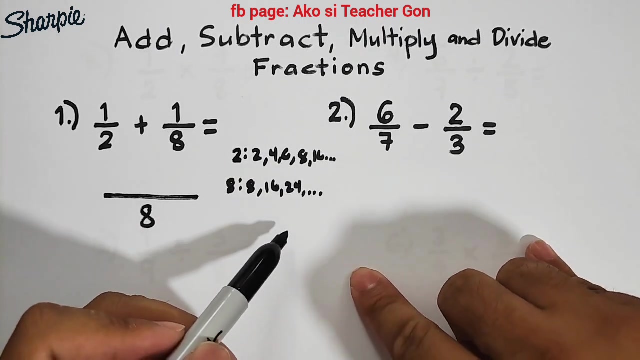 2, 4, 5, 6, 7, 8. 2, 4, 6, 8, 16, and so on. We are just listing the multiples of 2 and 4, 8. So, we have 8, 16, 24, and so on. As you can see, we have common multiples here, which is 8. Yes, sir, we also have 16. Ah, that's not it, because our target here is to get the least common multiple, which is equal to 8. And then, this least common multiple is 8. And then, this least common multiple is 8. 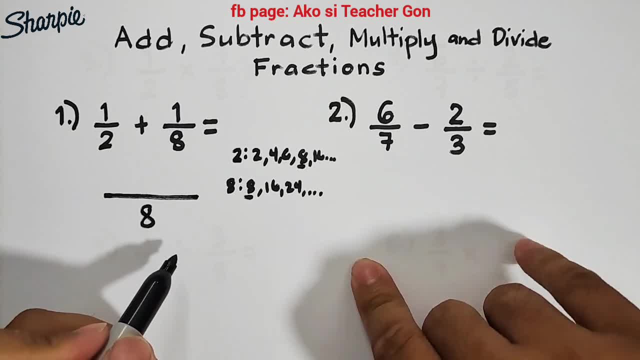 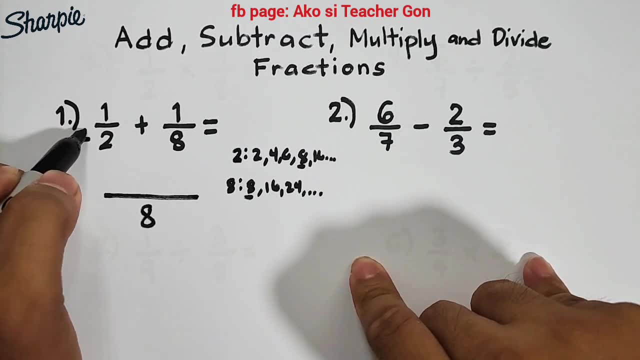 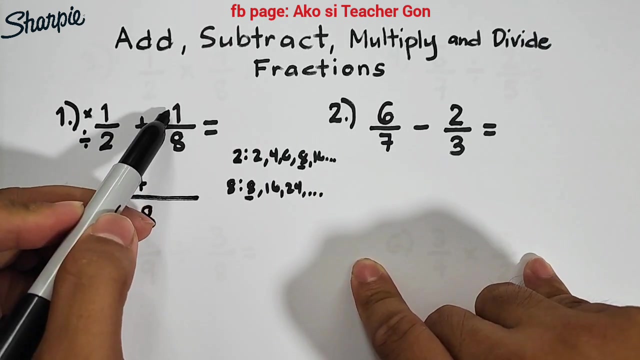 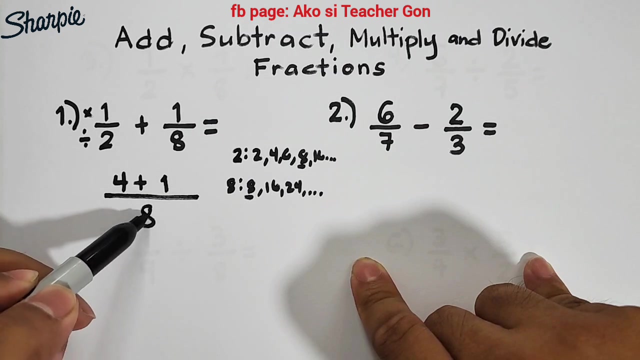 So, 8 will serve as your LCD, or your least common denominator. So, what's next is, this least common denominator, we need to divide it here in the original denominator, which is 8 divided by 2, that is equal to 4, and then multiply. 8 divided by 2 is 4, times 1, we have now 4. Plus, 8 divided by 8, which is equal to 1. Plus, 8 divided by 8, which is equal to 2, times 1, that is equal to 1. Again, let me repeat the process. First, you will divide this LCD to your original denominators, and then multiply it to the numerator. 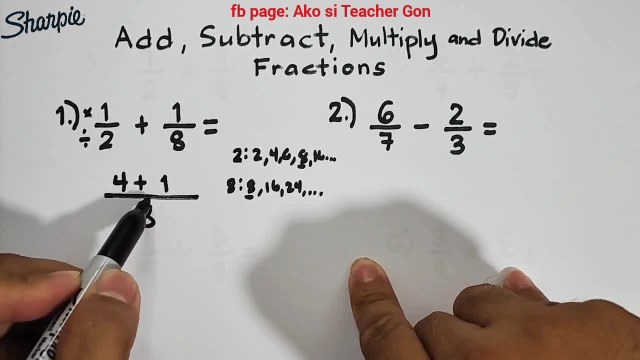 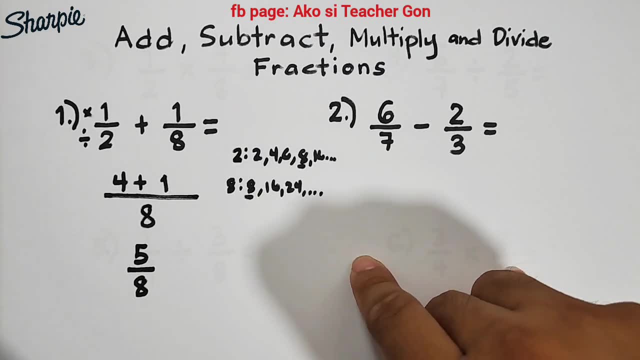 So, what we have now is 4 plus 1 over 8, and we need to simplify this, and the answer here is 5 over 8. By the way, guys, before declaring that your answer is the final answer, you need to check if the given fraction is already in simplified form. 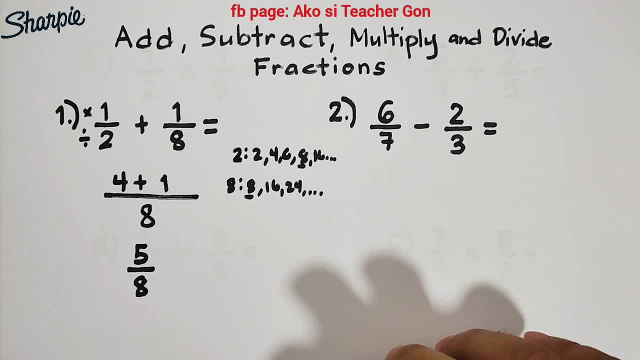 So, how will we know if it's already simplified, if it doesn't have a common factor? Okay? 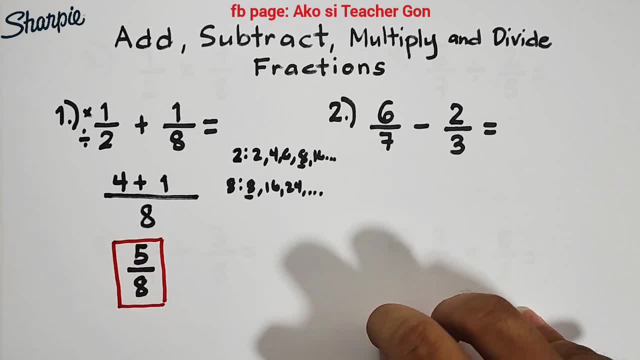 So, therefore, this is the final answer. We have 5 over 8. 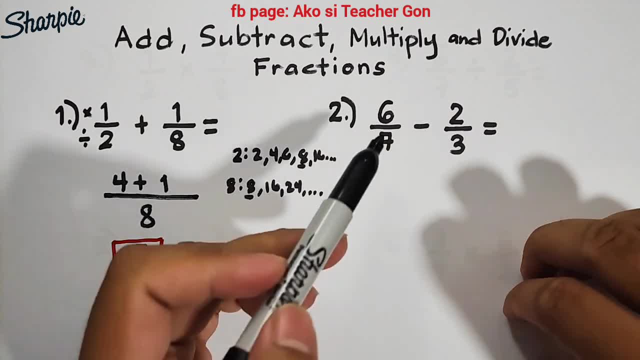 Now, let's move on with item number 2. For number 2, we have 6 over 7 minus 2 over 3. As you can see, we have different denominators again. 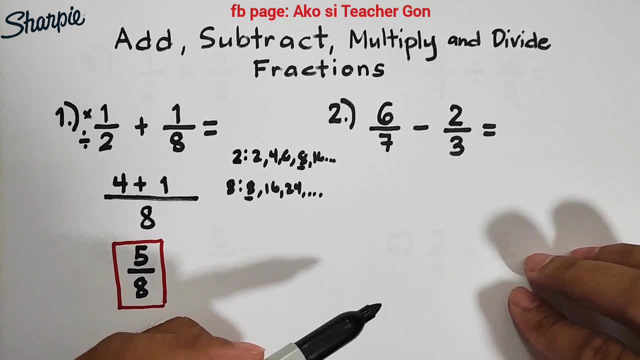 So, primarily, we need to find the LCD. Okay? 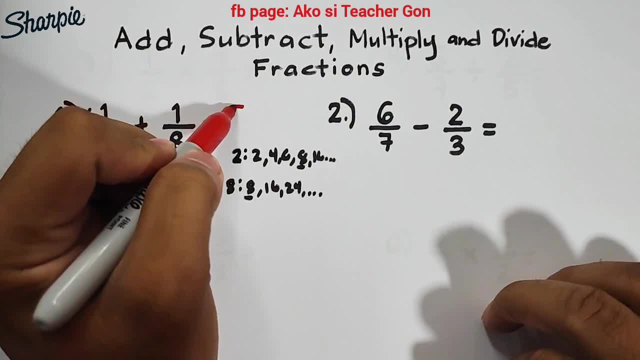 So, by the way, I need to write the answer here, which is 5 over 8. So, let's continue. 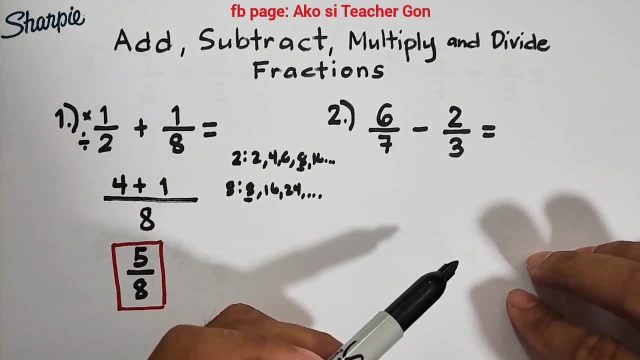 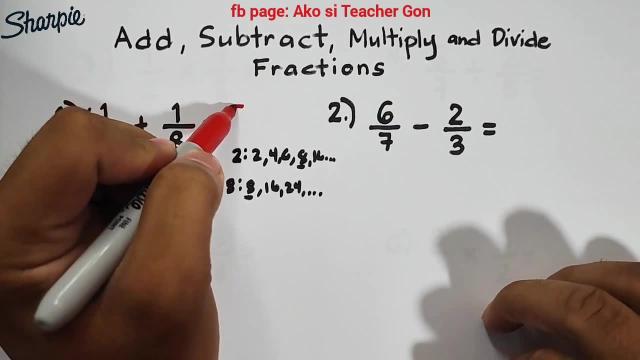 As you can see, we have different denominators again. So primarily we need to find the LCD. Okay, So, by the way, I need to write the answer here, which is 5 over 8.. So let's continue. 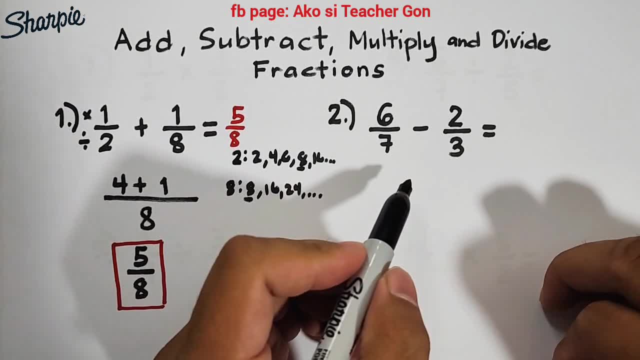 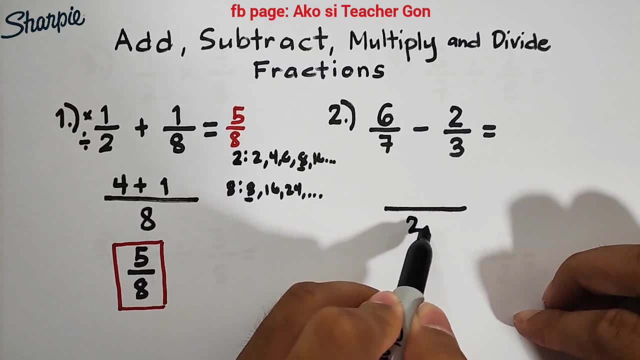 Our denominators are 7 and 3.. So, knowing the LCM, which is 21,, so our LCD is 21.. So let's repeat the process: Divide, multiply 21, divided by 7.. It's 3 times 6.. 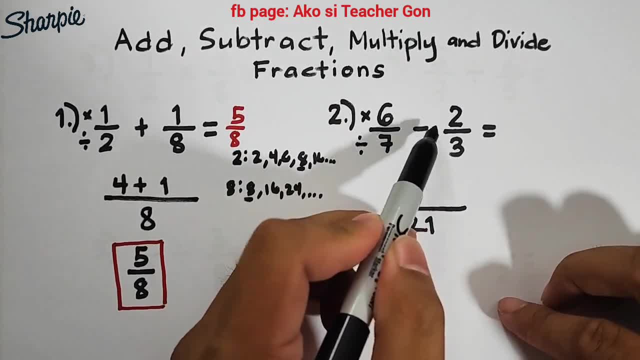 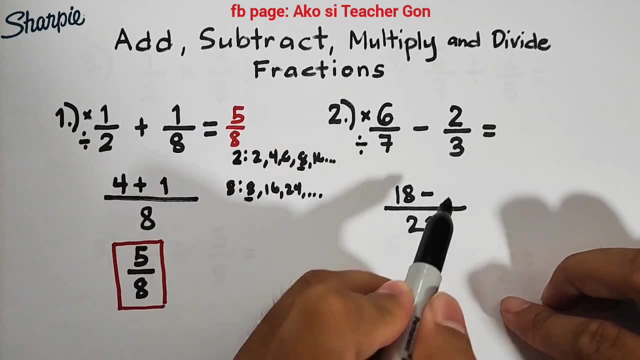 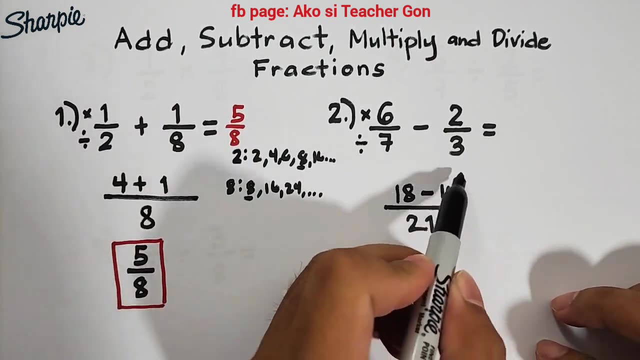 That is equal to 18.. And then copy this operation: minus 21 divided by 3.. That is 7.. Again, 21 divided by 3 is 7 times 2,, which is equal to 14.. We need to simplify our numerator. 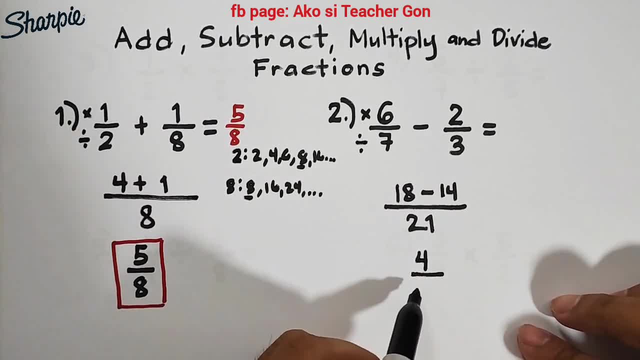 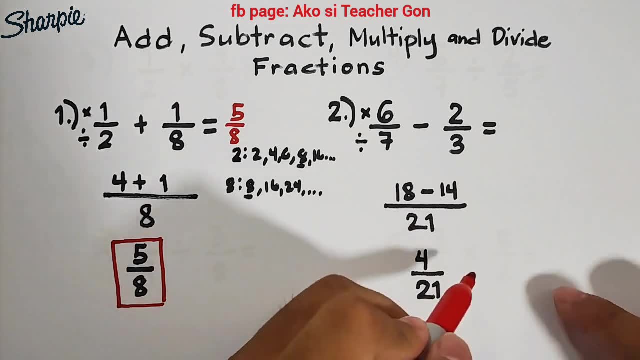 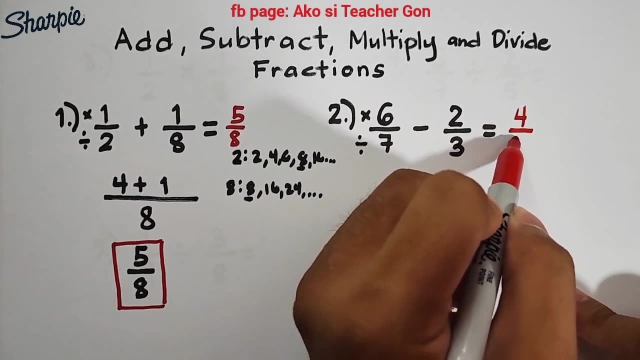 18 minus 14,, which is equal to 4 over 21.. This is now the final answer, guys. It's already simplified One more time: common factor: So we have 4 over 21.. And this is also 4 over 21.. 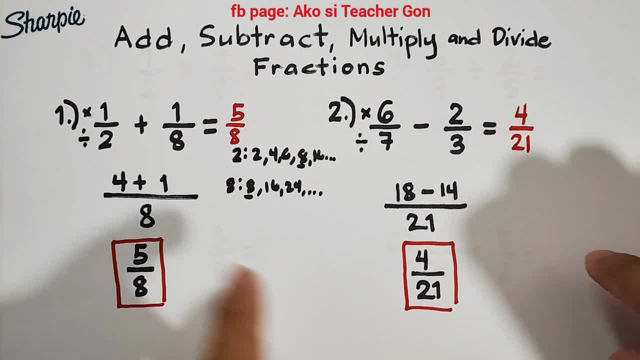 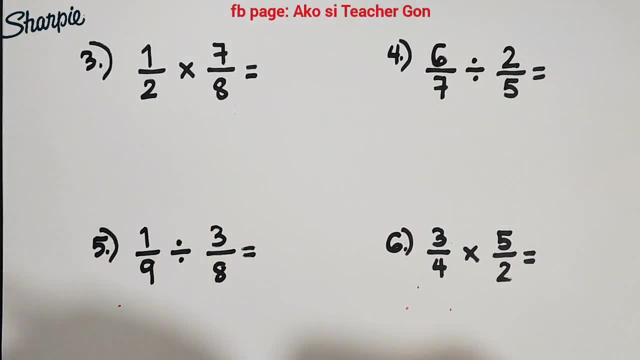 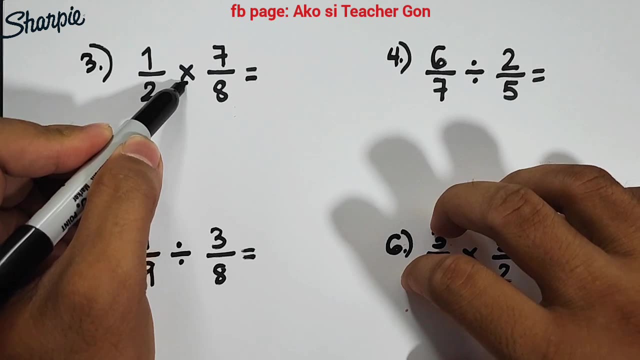 So we are done with addition and subtraction. So let us proceed with multiplication and division. So what we have here is item number 3.. For number 3, we are given 1 half times 7 over 8.. Remember, guys, there's a method of cancellation. 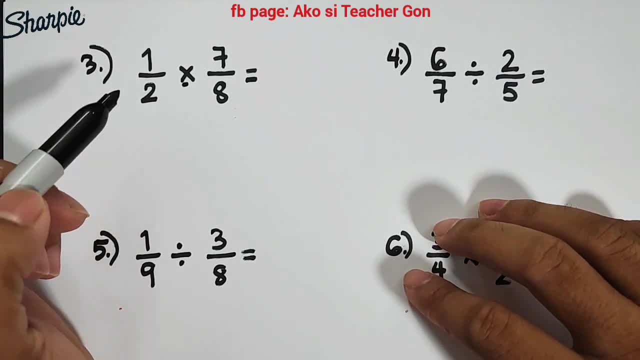 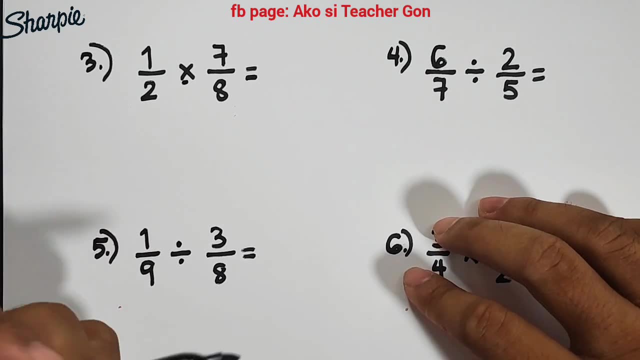 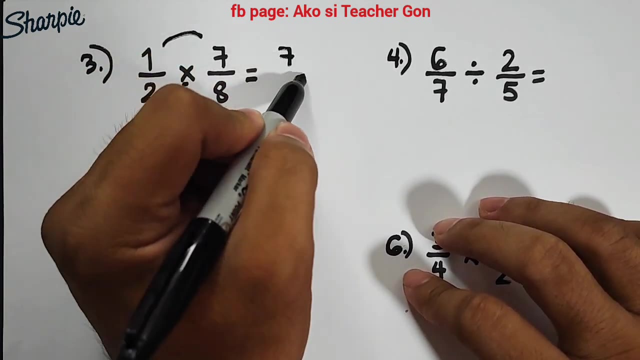 But what we will do here in number 3 is our common way, which is simply multiplying the numerators, and eventually we will simplify our answer. Here we have 1 times 7.. That is equal to 7 over 2 times 8.. 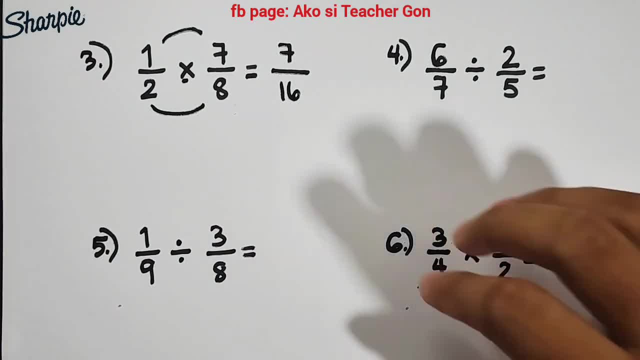 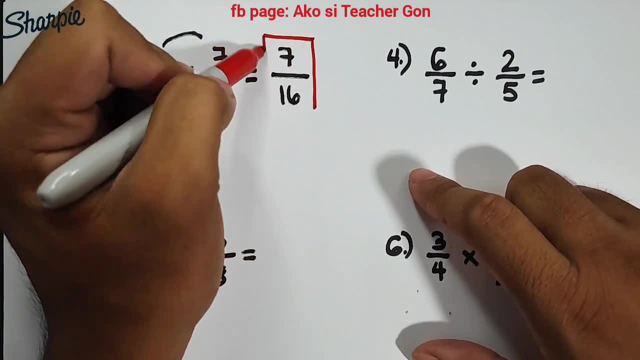 That is equal to 16.. If you are good with simplifying fraction, you already know that 7 over 16 is already in lowest term. So we will say that 1 half times 7 over 8 is equal to 7 over 16.. 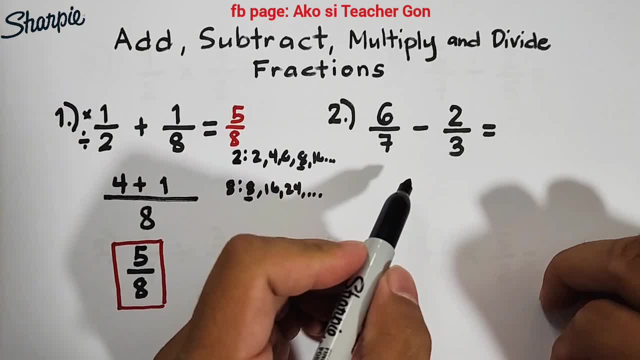 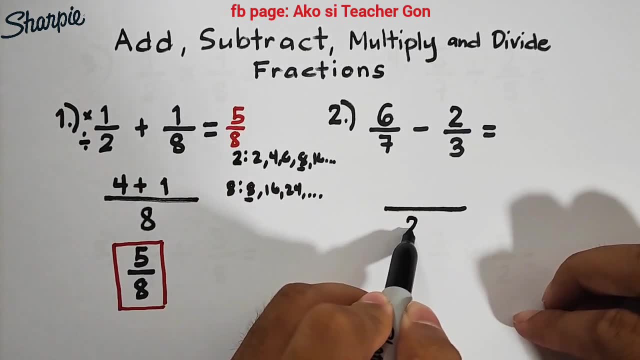 Our denominators are 7 and 3. So, knowing the LCM, which is 21, so our LCD is 21. 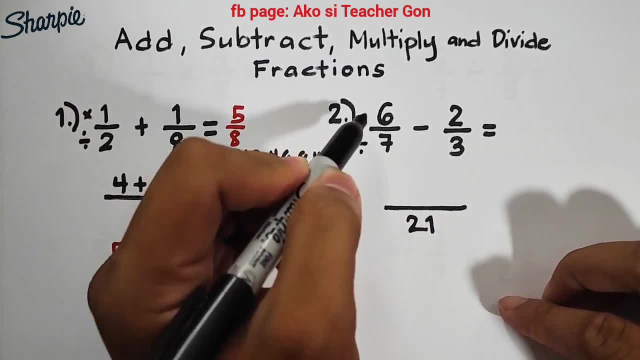 So, let's repeat the process. Divide, multiply. 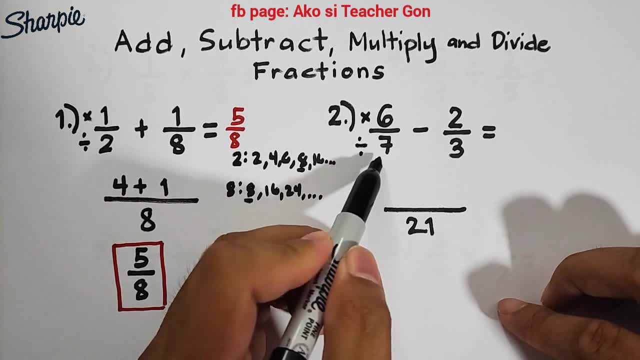 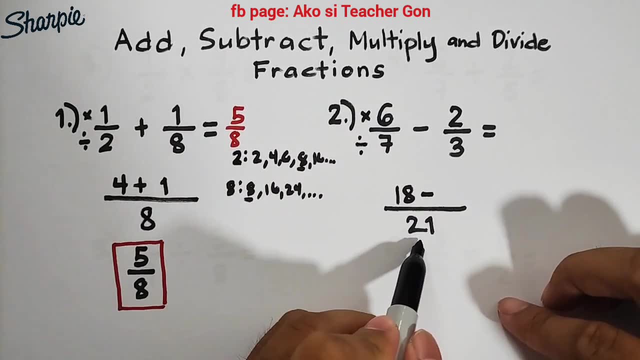 21 divided by 7 is 3. Times 6, that is equal to 18. And then copy this operation, minus 21 divided by 3, that is 7. 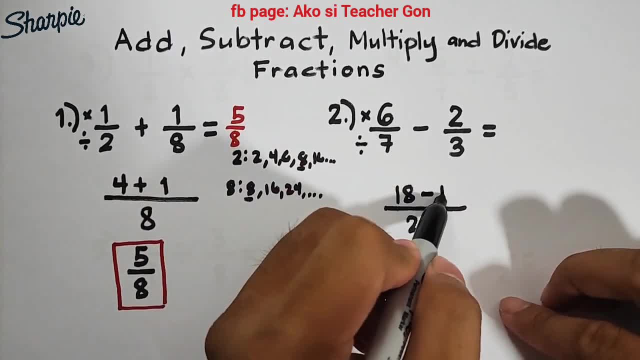 Again, 21 divided by 3 is 7. Times 2, which is equal to 14. 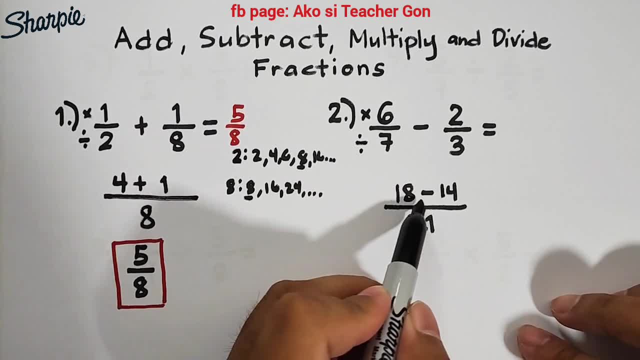 We need to simplify our numerator. 18 minus 14, which is equal to 4, over 21. This is now the final answer, guys. It's already simplified. 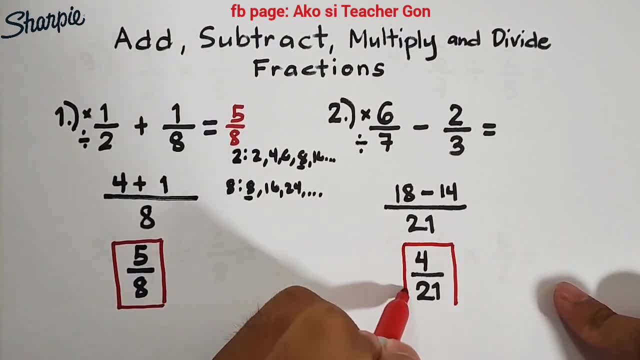 We have 4 over 21, and this is also 4 over 21. 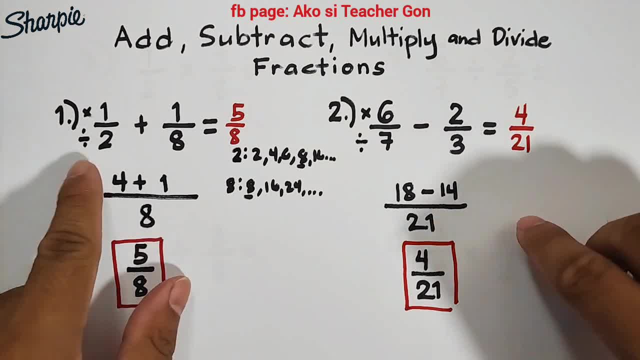 So, we are done with addition and subtraction. So, let us proceed with multiplication and division. 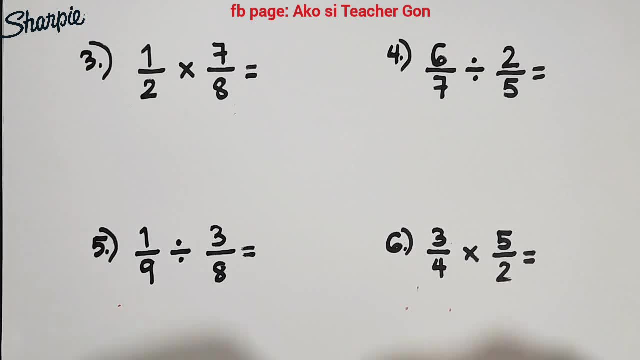 So, what we have here is item number 3. 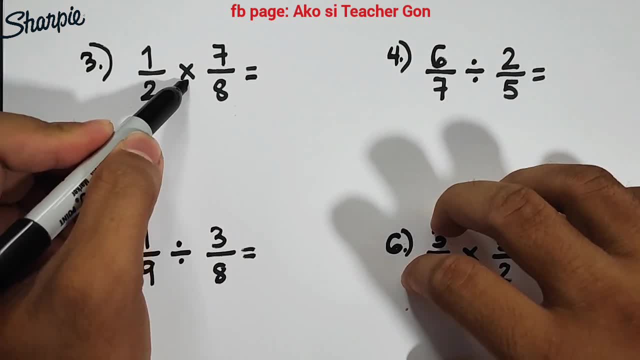 For number 3, we are given 1 half times 7 over 8. Remember, guys. 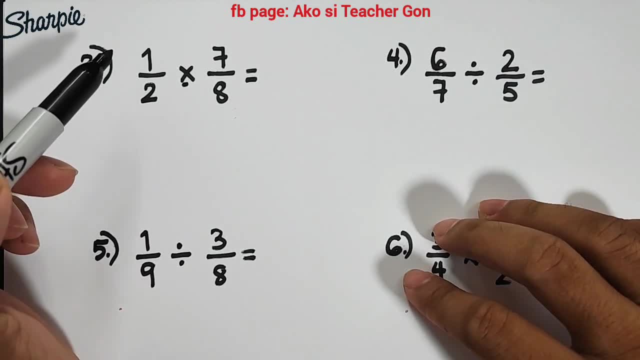 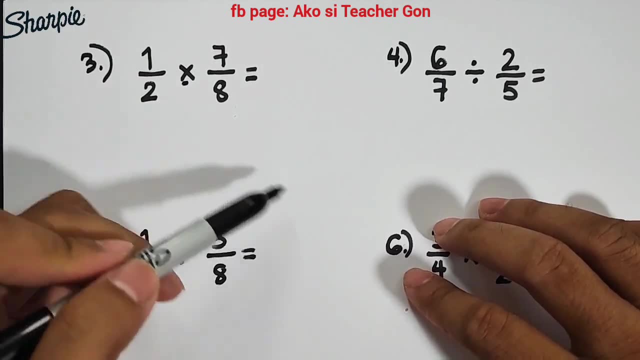 There's a method of cancellation. But what we are going to do here now, for number 3, is our common way, which is simply multiplying the numerators and numerators, and eventually, we will simplify our answer. 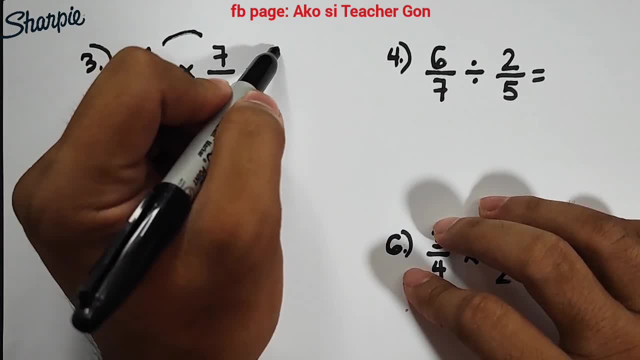 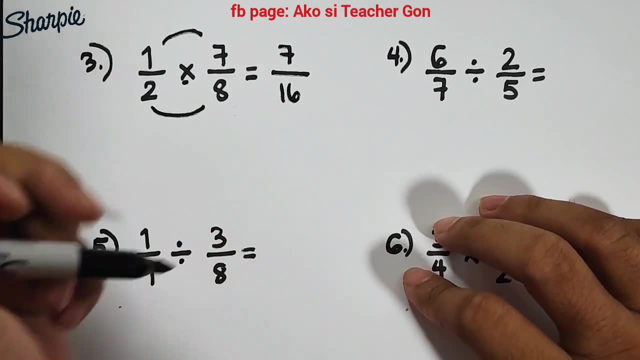 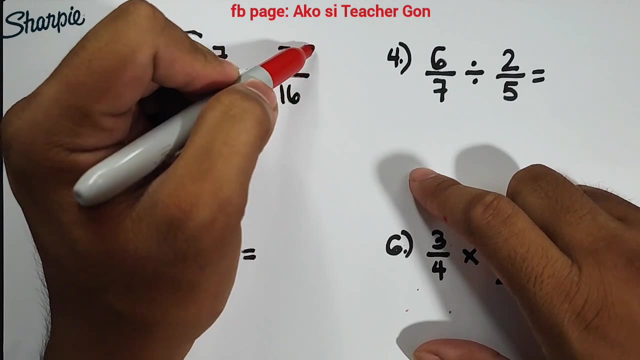 Here, we have 1 times 7, that is equal to 7, over 2 times 8, that is equal to 16. If you are good with simplifying fraction, you already know that, 7 over 16 is already in lowest term. 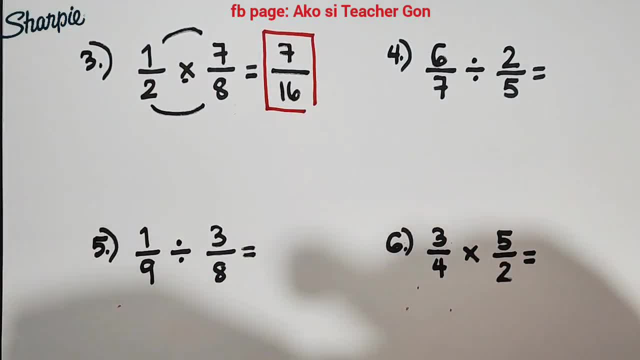 So, we will say that 1 half times 7 over 8 is equal to 7 over 16. Now, let's continue. 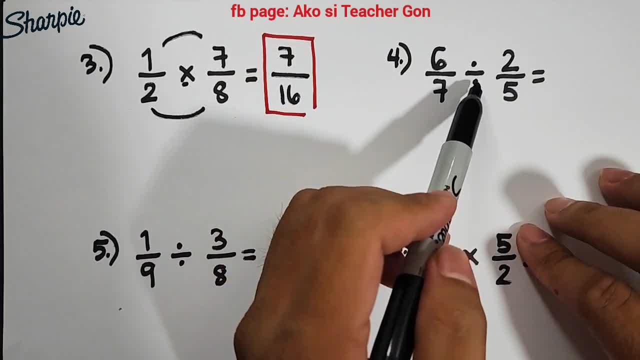 For number 4, this is division. We have 6 over 7 divided by 2 over 5. Okay? 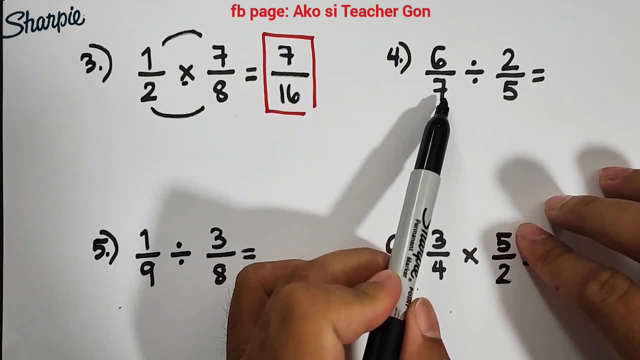 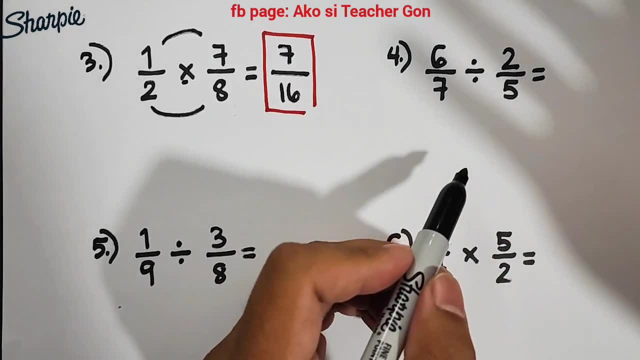 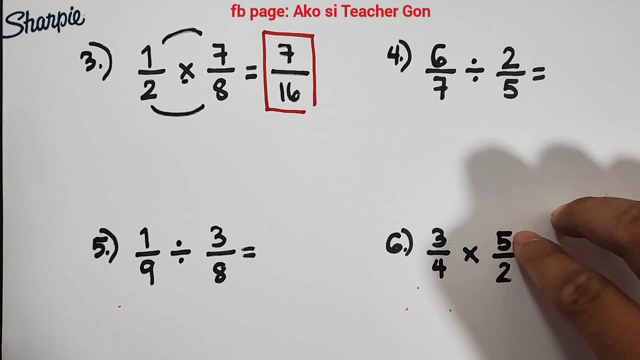 Now let's continue For number 4, this is division. We have 6 over 7 divided by 2 over 5.. Okay, So what we need here? remember this, guys. Okay For dividing fraction. you will go through multiplying fractions again. 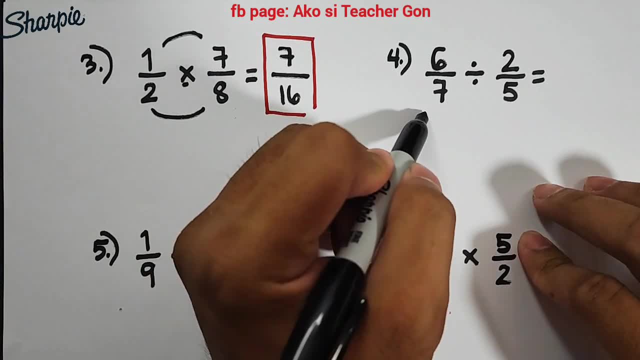 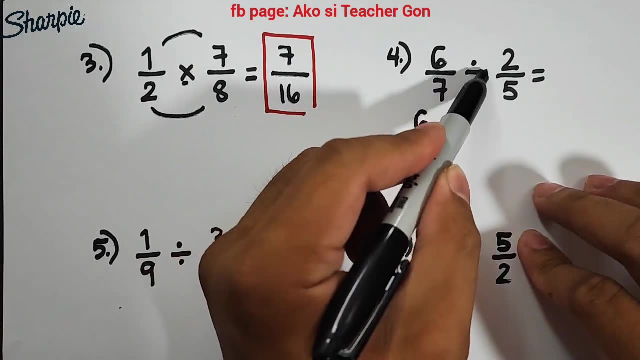 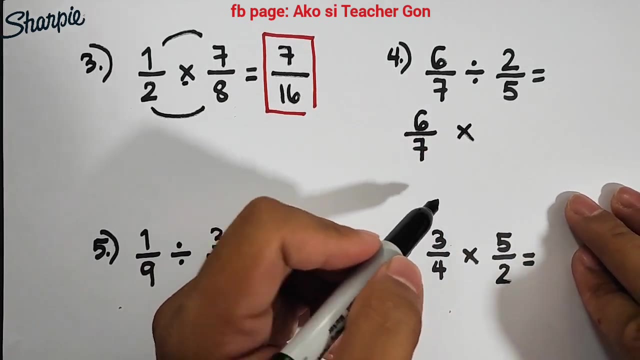 First we need to copy the first fraction. We have 6 over 7.. Again, copy the first fraction. Next, this division, symbol or operation. you will change this into multiplication. Next, you will find the reciprocal of 2 over 5, which is 5 over 6.. 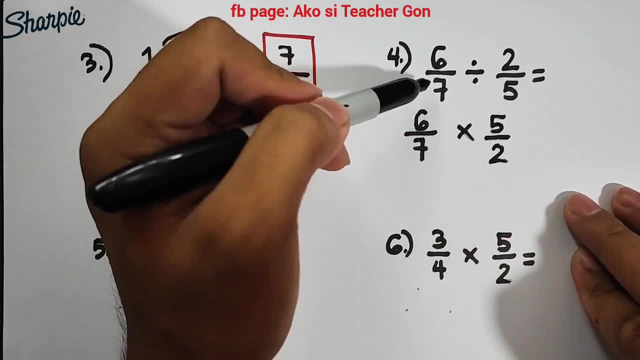 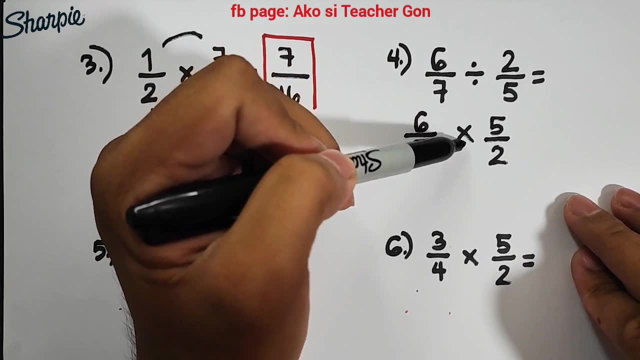 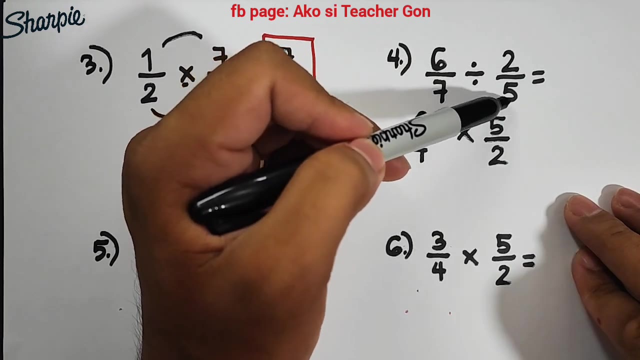 This is 5 over 2.. Again, copy the first fraction, This division symbol. you need to change this into multiplication symbol And then, for the second fraction, you need to get the reciprocal of it, which is 5 over 2.. 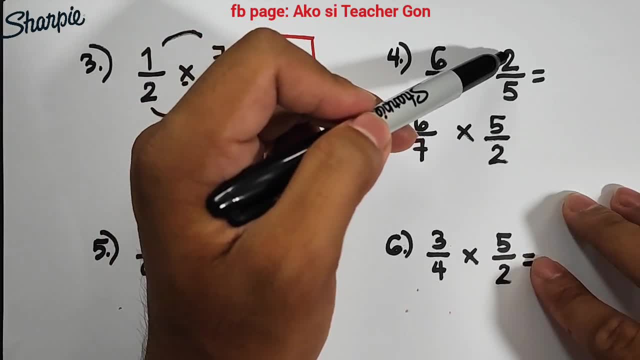 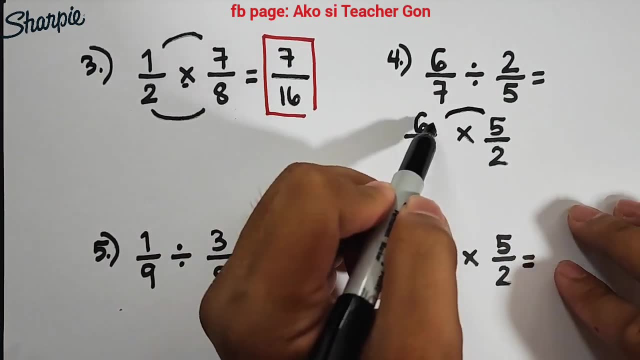 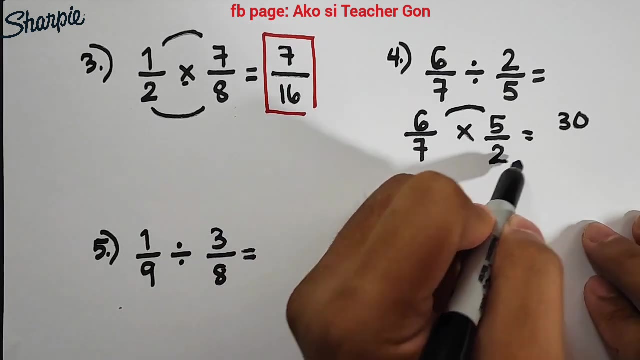 You will just flip it or you will interchange the position of your numerator and denominator And then go with multiplication. So we need to multiply this 6 times 5,, which is equal to 30. And then 7 times 2,, which is equal to 14.. 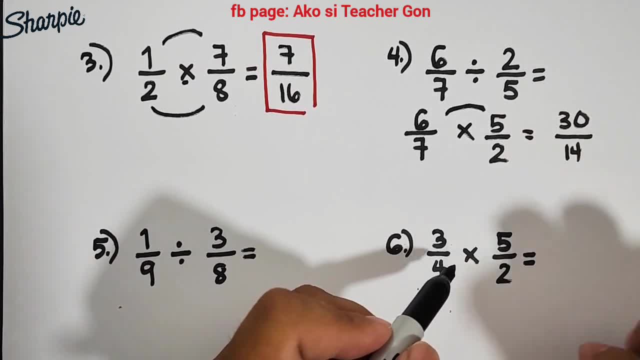 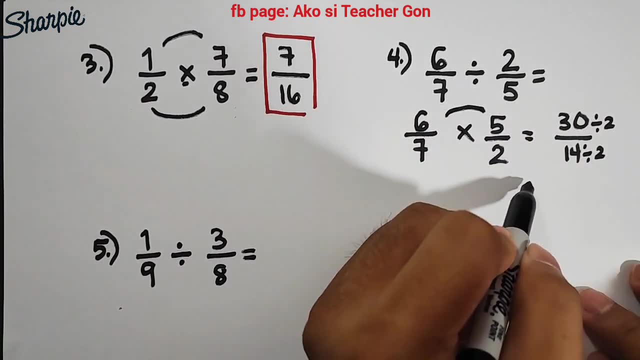 So, as you can see, the two numbers- 13 and 14, are both divisible by 2.. So we can divide this by 2.. Okay, And then, as you can see, 30 divided by 2 is 15.. 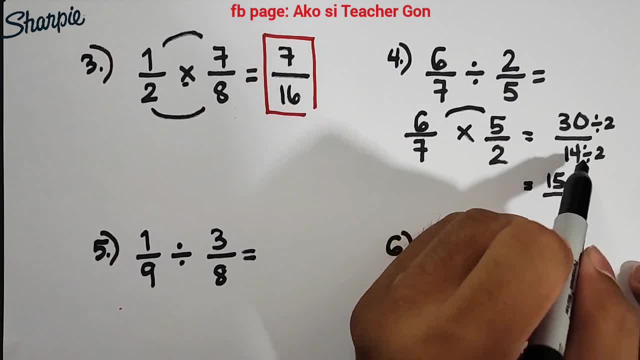 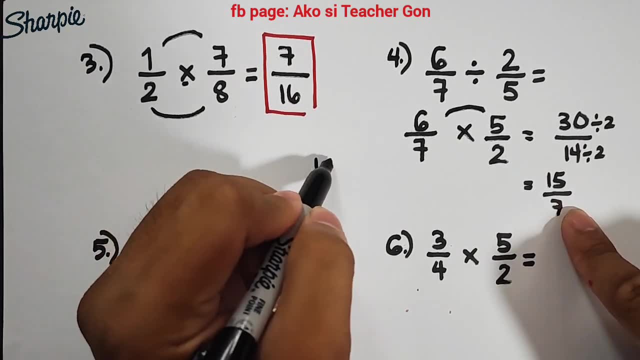 Over 14 divided by 2.. 14 divided by 2, which is equal to 7.. By the way, guys, we can also convert this into mixed number. Sir, how do we do that? Just like this: 15 divided by 7.. 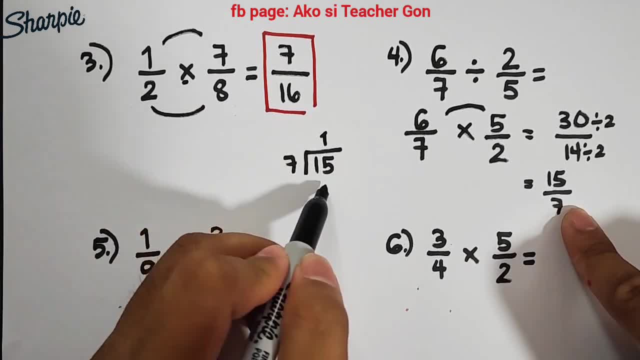 15 divided by 7 is 1.. 1 times 7 is- Oh sorry. 15 divided by 7 is 2.. 2 times 7 is 14.. And then you will subtract this. We have 1.. 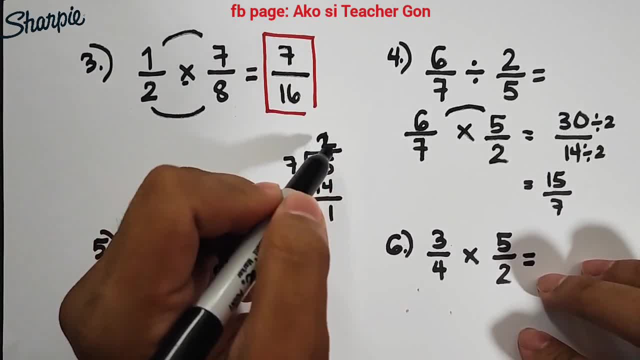 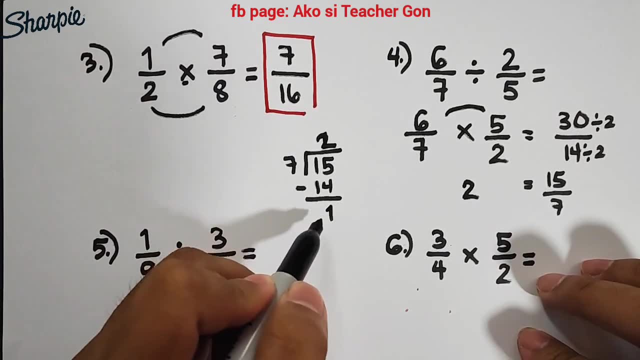 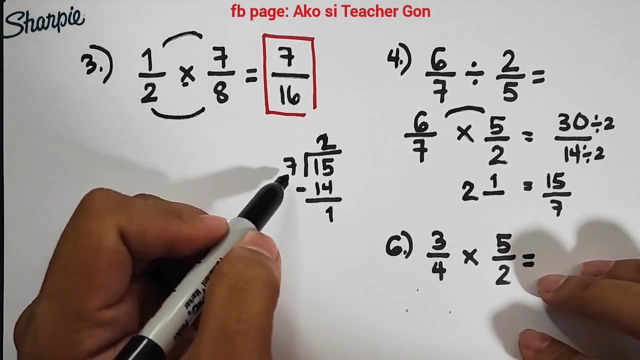 So here now our quotient is 2.. Okay, That will serve as your whole number in the mixed number, And then this is your remainder 1. You will put it here in your numerator And then for the denominator you will copy the original denominator of your 15 over 7.. 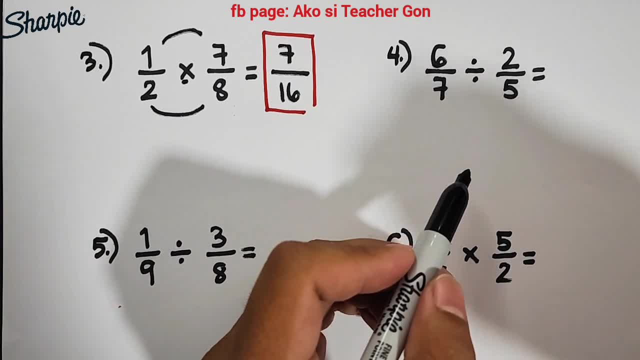 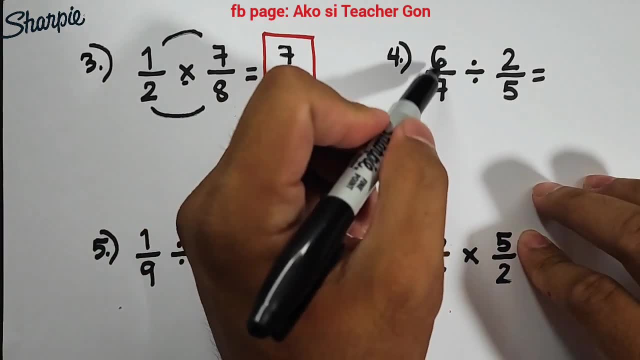 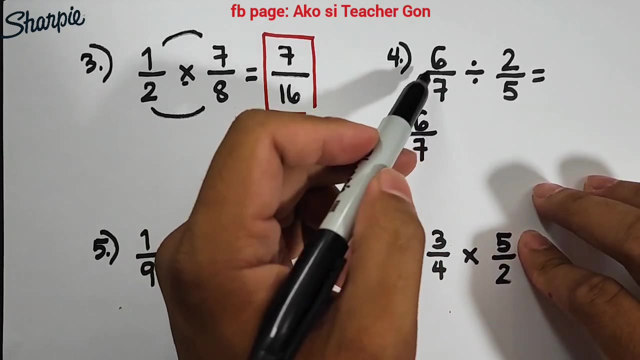 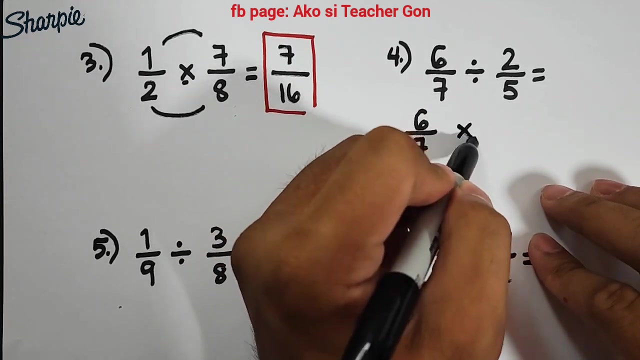 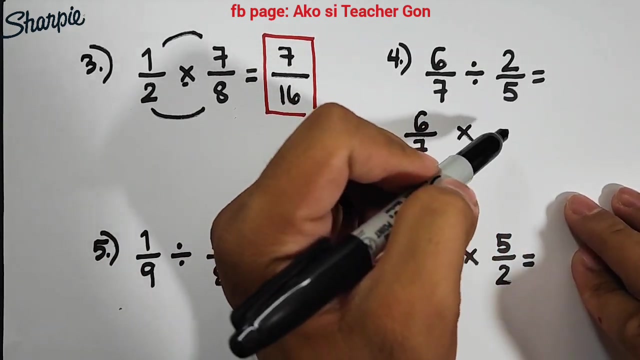 So, what we need here, remember this, guys. When you're dividing fraction, you will go through multiplying fractions again. First, we need to copy the first fraction. We have 6 over 7. Again, copy the first fraction. Next, this division symbol or operation, you will change this into multiplication. Next, you will find the reciprocal of 2 over 5, which is 5 over 2. Again, copy the first fraction. 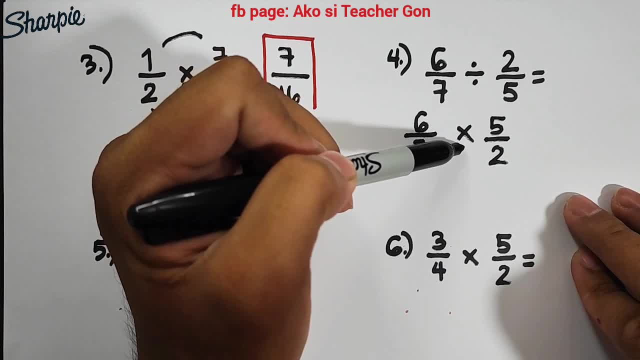 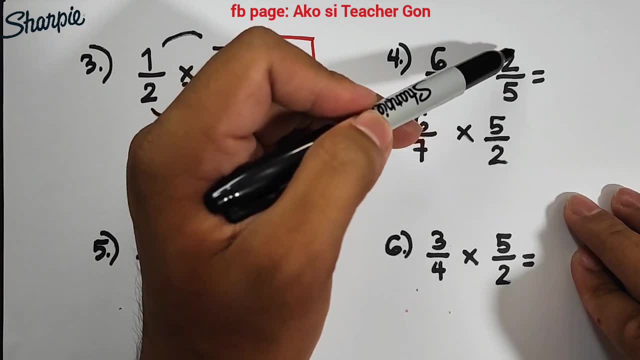 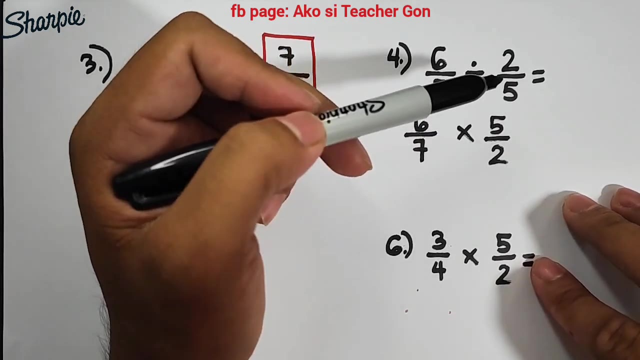 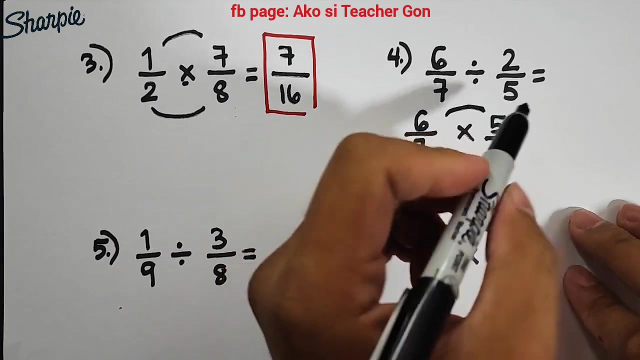 This division symbol, you need to change this into multiplication symbol. And then, for the second fraction, you need to get the reciprocal of it, which is 5 over 2. You will just flip it. Or you will interchange the position of your numerator and denominator. And then, go with multiplication. So, we need to multiply this. 6 times 5, which is equal to 30. 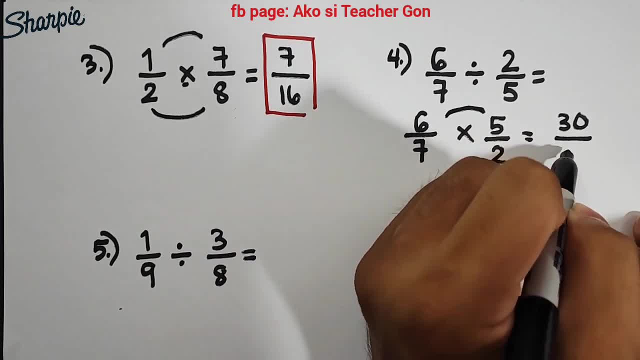 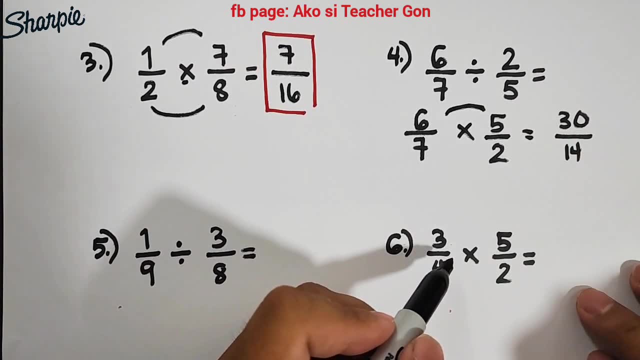 And then, 7 times 2. Which is equal to 14. So, as you can see, the two numbers, 13 and 14, are both divisible by 2. So, we can divide this by 2. Okay? 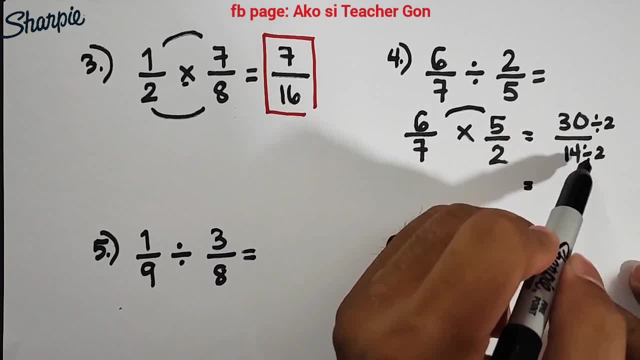 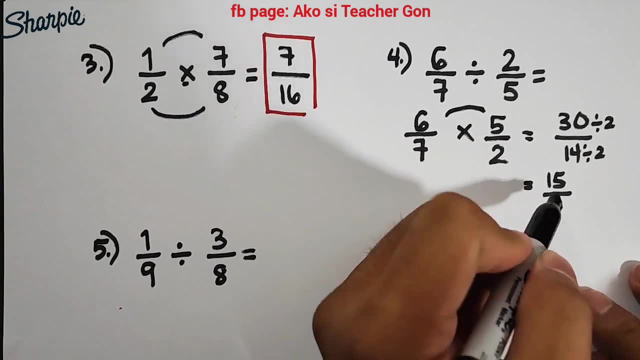 And then, as you can see, 30 divided by 2 is 15 over 14 divided by 2, which is equal to 7. By the way, guys, we can also convert this into mixed number. Sir, how do you do that? Just like this. 15 divided by 7. 15 divided by 7 is 1. 1 times 7 is... Ah, sorry. 15 divided by 7 is 2. 2 times 7 is 14. And then, you will subtract this. 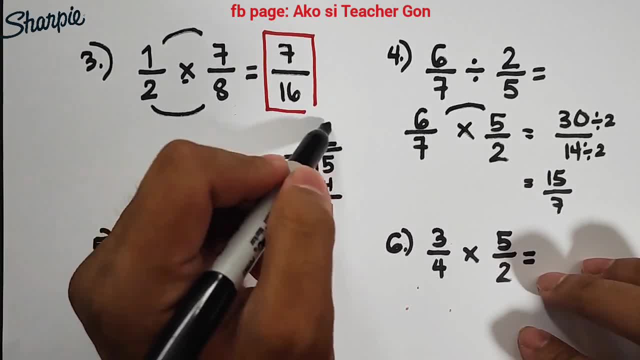 We have 1. So, here, our quotient is 2. 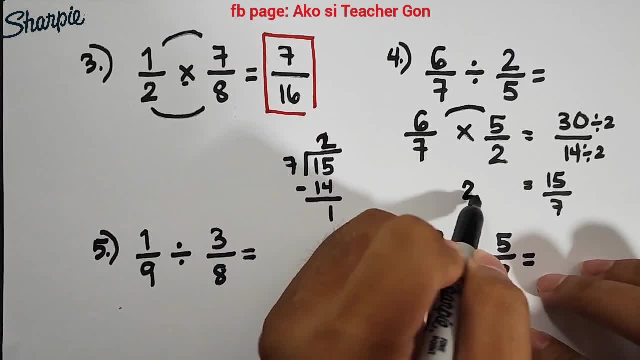 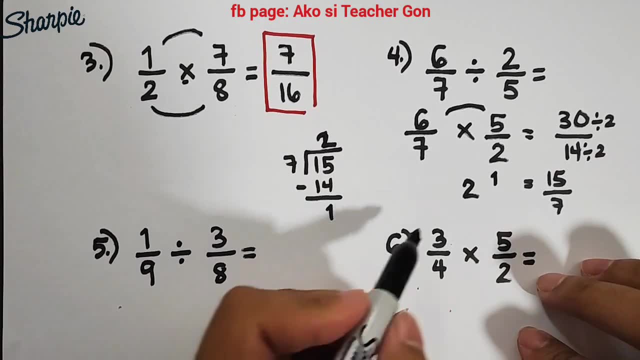 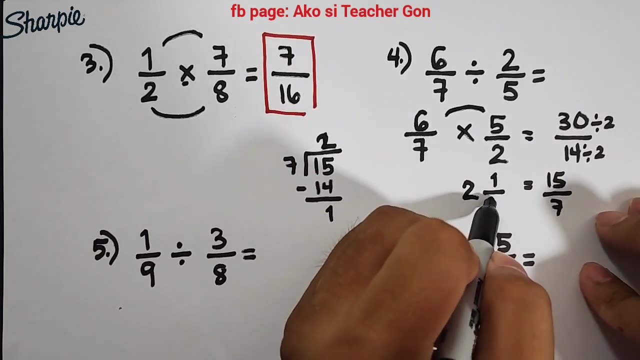 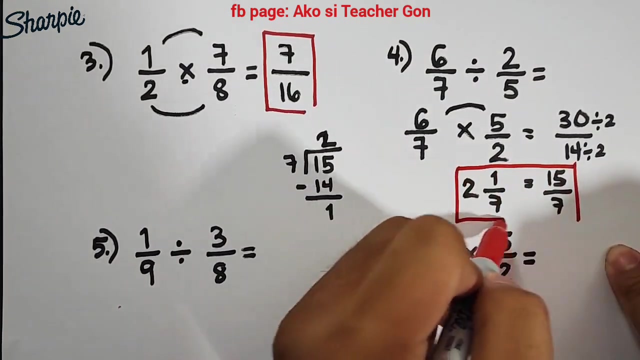 Okay? That will serve as your whole number in mixed number. And then, this is your remainder, 1. You will put it here in your numerator. And then, for the denominator, you will copy the original denominator of your 15 over 7. That's why, the correct answer here is 2 over 7 or 15 over 7. Either of the two is okay. 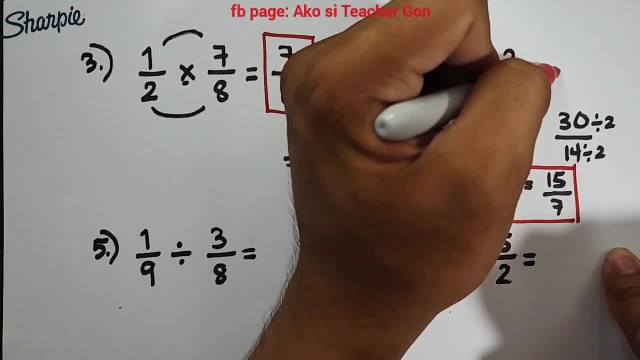 But, I will just write 2 and 1 over 7. 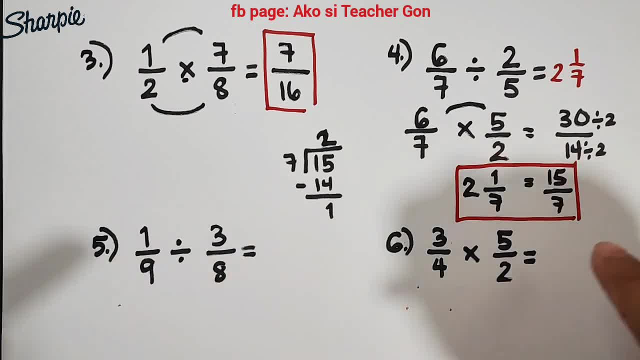 Sir, why is this 15 over 7 accepted? Because they are equal. 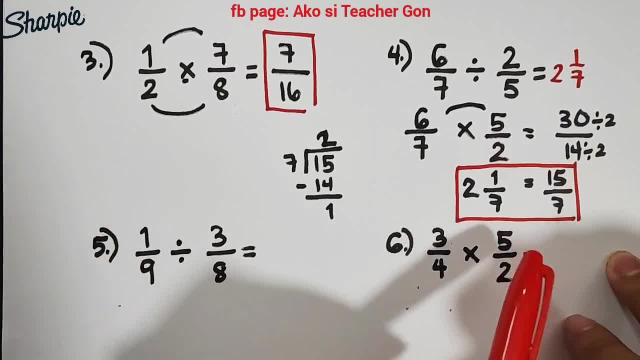 Some of the teachers are not asking the students to convert their final answer in mixed number. So, that's also okay. 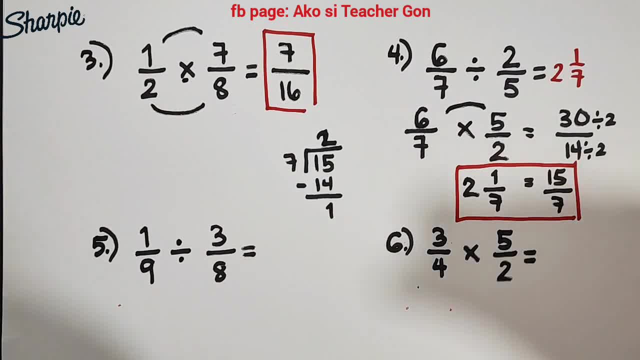 Now, guys, I hope that you learned in our video on how to add, subtract, multiply, and divide fractions. 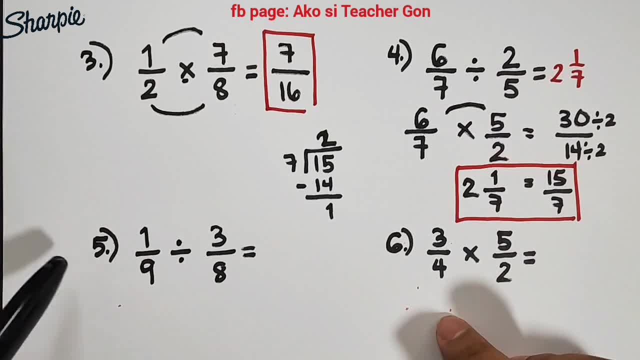 Now, it's your turn to answer number 5 and number 6. 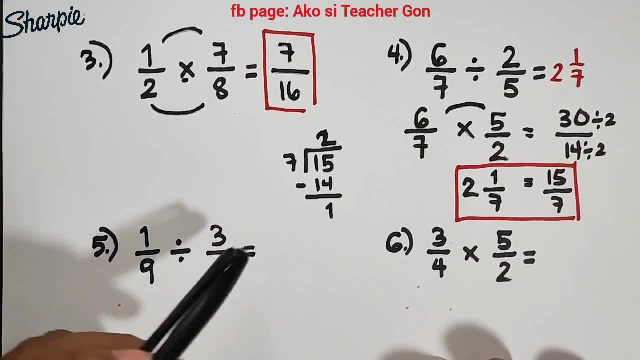 In number 5, we are given 1 over 9 divided by 3 over 8. 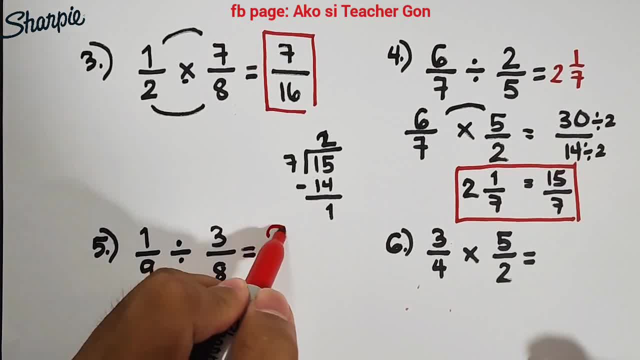 In number 6, okay? In number 6...